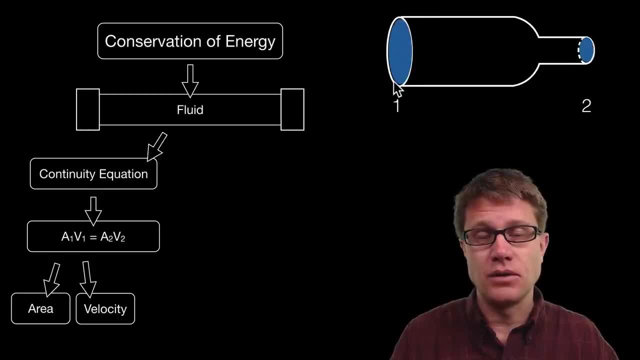 is going to be the area over here, And so if we look at the velocity, that is what V1 stands for. Since we have a large cross sectional area here, we are going to have a relatively low velocity And then, as we move to the right, since we are decreasing that area, we are going 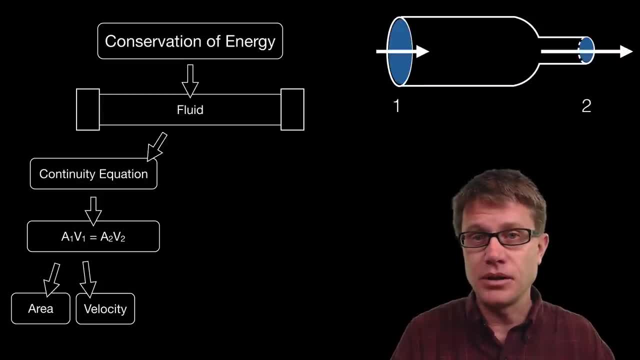 to have a high velocity, And so if you know the velocity at any point in the pipe, since that whole fluid is moving, if you know the cross sectional area anywhere else, you are going to be able to figure out the velocity. An application of this: if you have ever had a hose as water comes out of it, it has. 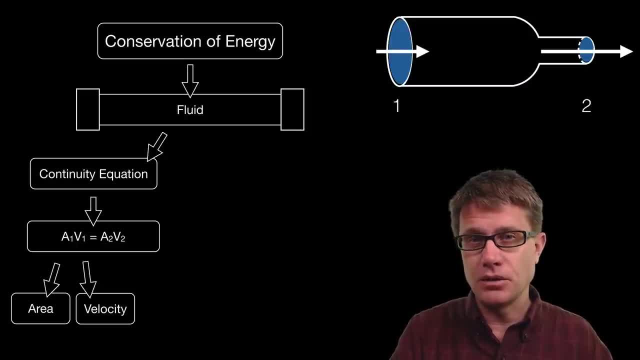 got a large cross sectional area. If you put your thumb in front of it, what are we doing? We are decreasing the cross sectional area. What happens to the velocity It increases? Now, if we look at Bernoulli's equation, it is somewhat scary when you see it. the first: 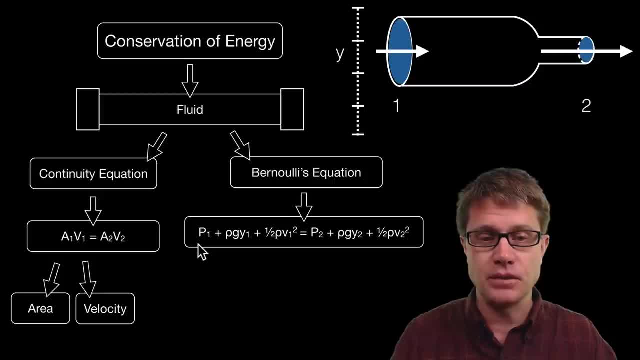 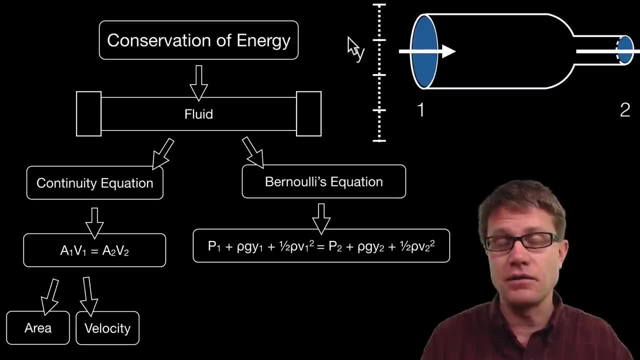 time It looks like this, And so this is going to be Bernoulli's equation And it is frightening to look at. But what we have really added here are simply two things. We have added y, which is going to be the height of the pipe, Because that is the potential velocity. 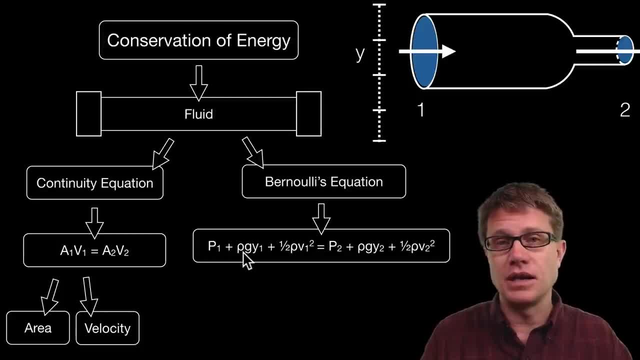 The potential energy. And then the other thing we have added is a rho, which is going to be the density of the fluid, Because those can affect the amount of energy that we have. And so if we break apart this equation, we have also got 1 on the left side and 2 on 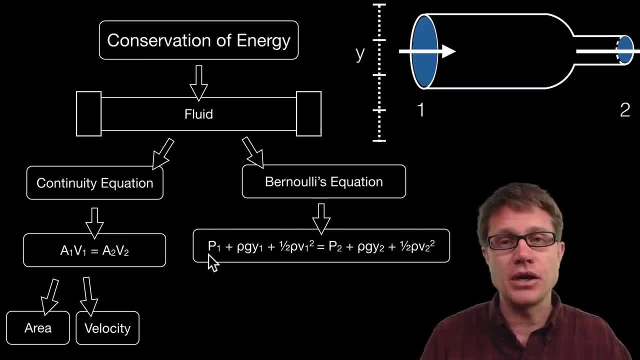 the right side. If we look at this first one, p1 stands for the pressure, So inside the fluid itself. how much is that fluid pushing in on a point inside the fluid itself? So that is going to be the pressure energy. We then have this rho g, y1, which is going to 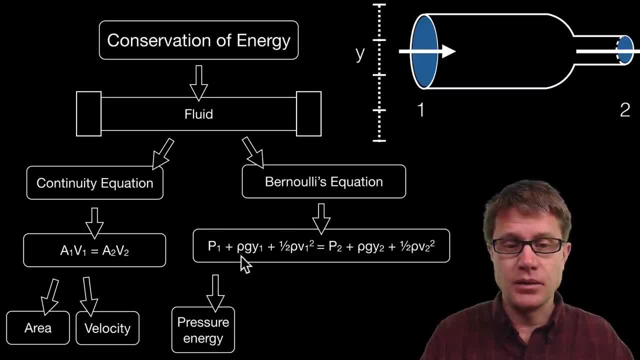 be the density of the fluid. Now, that seems confusing, But let me kind of write it out a different way. If we were to, instead of writing rho or density, if I were to say the mass, this is g, gravitational energy or gravitational field strength. And then if we were to look 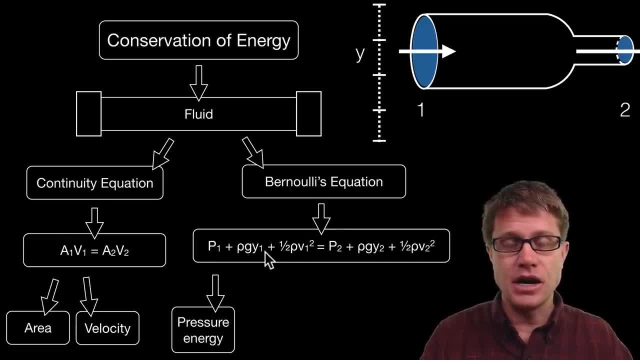 at y, if I wrote H there, or the height, what is m, g, h? You know that That is just the potential energy of the fluid, And so that second bit of this equation is going to be the potential energy of the fluid. And then, if we write this next one, what is 1 half? 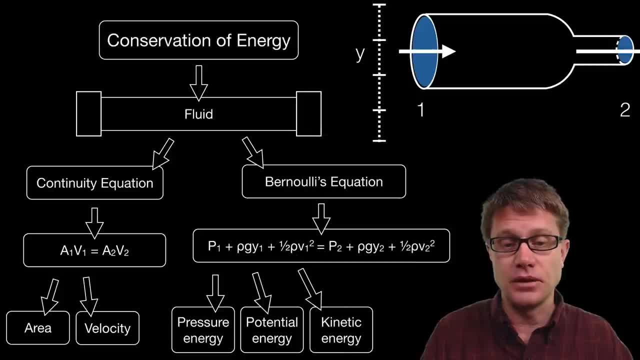 mv squared, That would be kinetic energy, But we are writing density ofوم hated the density, since we are dealing with a fluid. So that is going to be the kinetic energy, And so those are the three ways we can get energy. on the left side of that pipe It is. 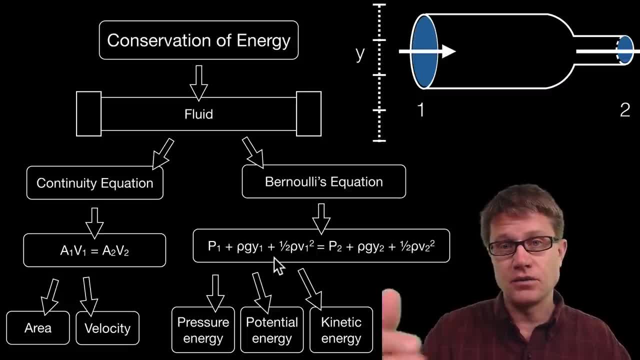 the pressure of the fluid, It is the potential energy, how far it is in relation to gravity, And then the last is going to be the speed of that fluid. And since this is the conservation of energy in these two points of the pipe, since we know the energy over here and we 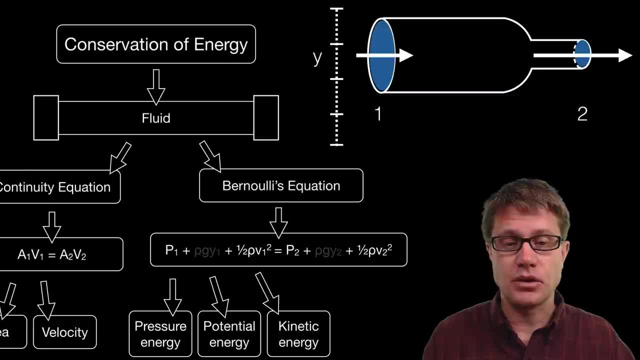 know it is going to be an equal amount of energy over here we can solve some pretty complex problems. So, for example, if we were to look at this pipe right here, on both sides they both have the same height or the same y value. So I have taken those out of this. 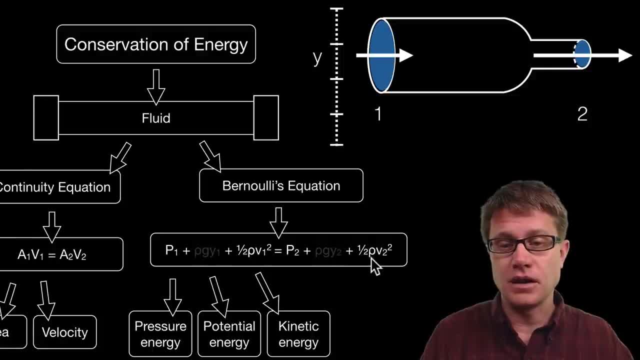 equation. And so where is the velocity going to be faster? It is going to be faster on the right side of the pipe. So we are going to have a faster velocity on the right side, Slower velocity on the left side. So what has to be our pressure on the right side? 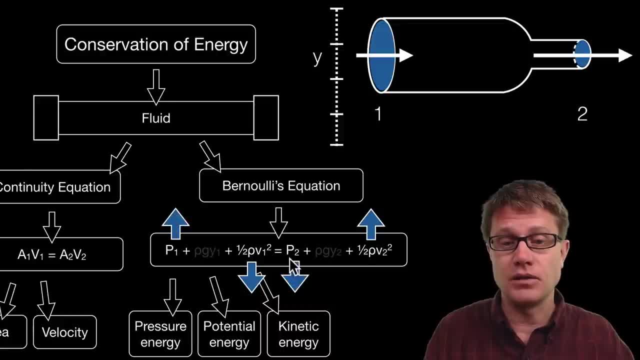 Well, to make it equal on either side- conservation of energy- we are going to have to have a lower pressure. So, just like in my example of the ship, if the fluid is moving fast, then it is going to have a lower pressure. And so let's start. 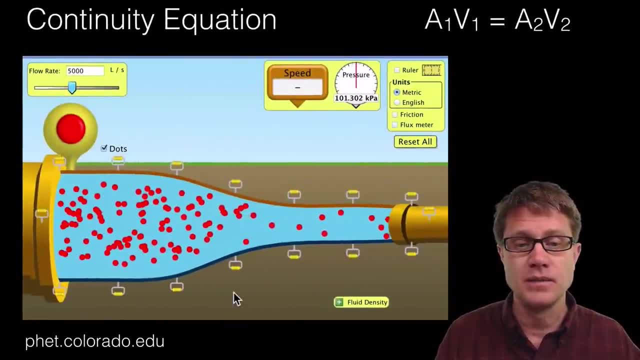 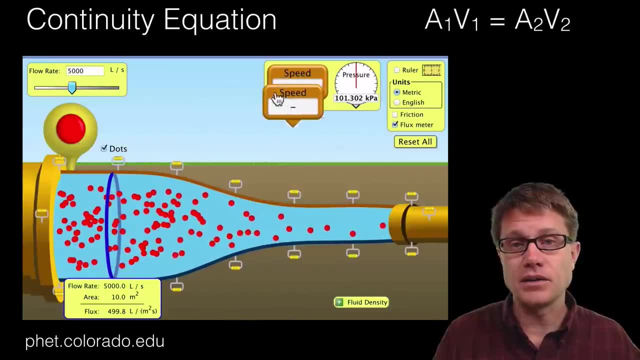 with the continuity equation, which is simple. We have got a PHET simulation. You can see as the fluid is moving. it is moving faster on the right, And so if we use a flux meter on the left side, the cross sectional area is 10 meters squared and the speed is going. 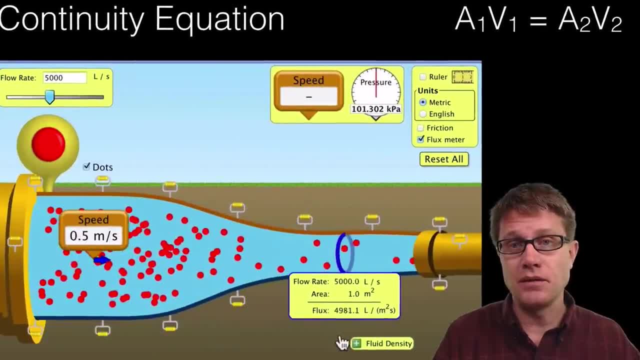 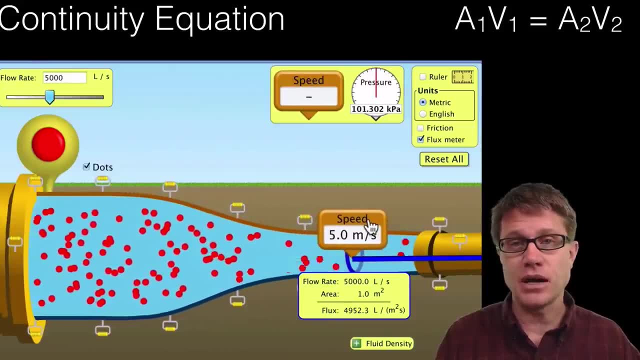 to be 0.5 meters per second. So that would be my A1 times my V1.. If I move over to the right side now, my cross sectional area is 1.. What is my velocity? 5 meters per second. 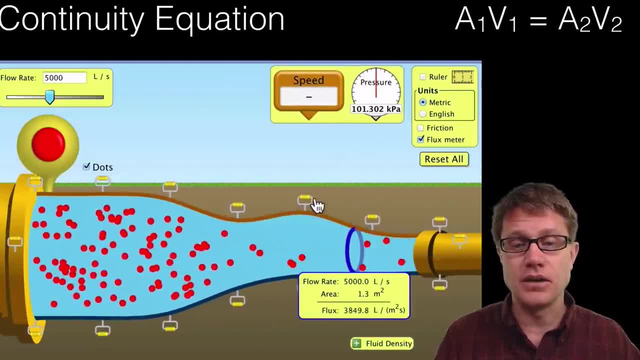 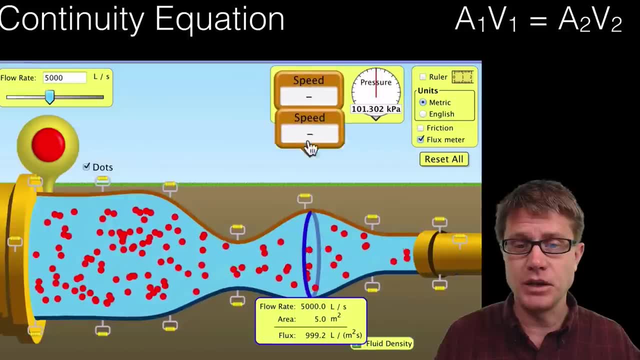 So I can just solve for the one. I do not know, and I can figure that out. If we were to just change the pipe now, the cross sectional area is 5 meters squared. What is going to be my speed? It is simply going to be 1 meters per second, And so continuity equation is very 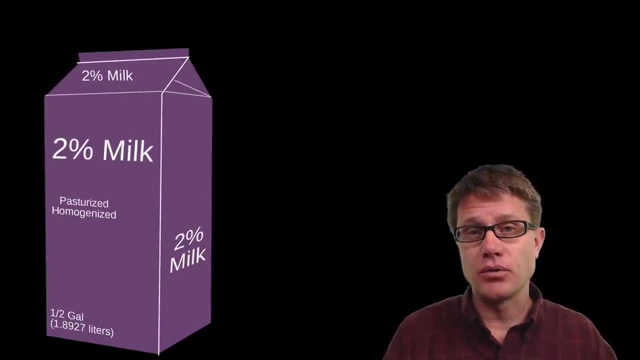 very simple. If we were to apply Bernoulli's equation, what we are really adding to it is the density of the fluid and then the height of the fluid. And so let me give you a thought experiment. Let's say we were to take a half a gallon of milk and I were to pop three holes. 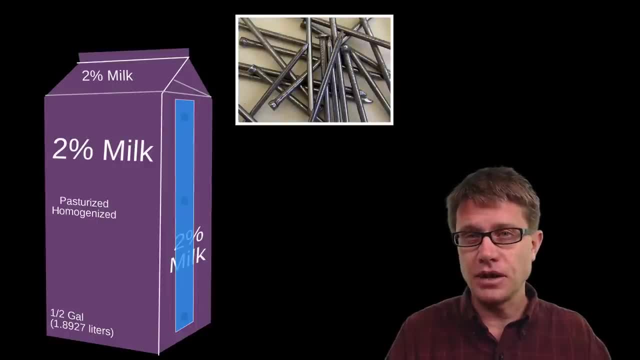 in it and quickly put tape in it. Well, that would be 0.5 meters per second. Now let's see if we can solve for the one. I do not know, and I can figure that out- If we were to apply tape over it like that, So the whole thing is filled up with a fluid. And then I were. 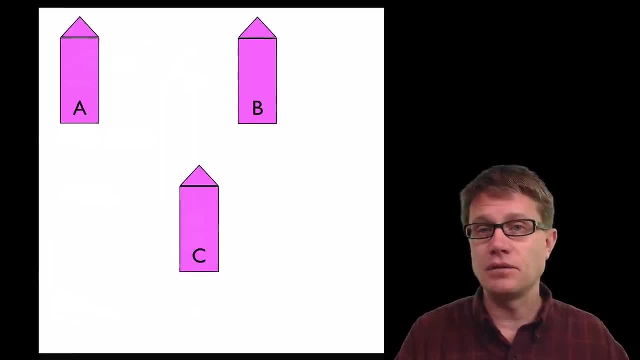 to simply pull the tape off the side. So what are we going to get? Streams of milk coming out of the carton. But do you think those streams would look like this, like this or like that if you were to look at it from the side? Which is going to be the correct way? 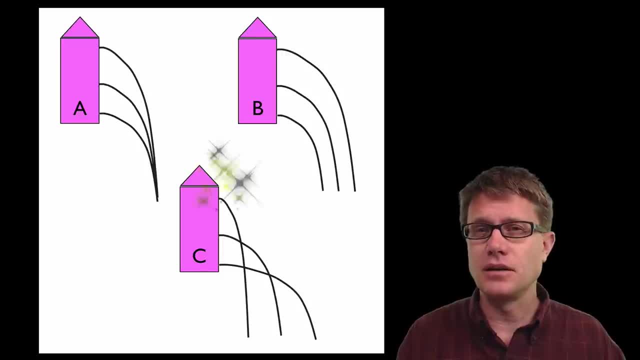 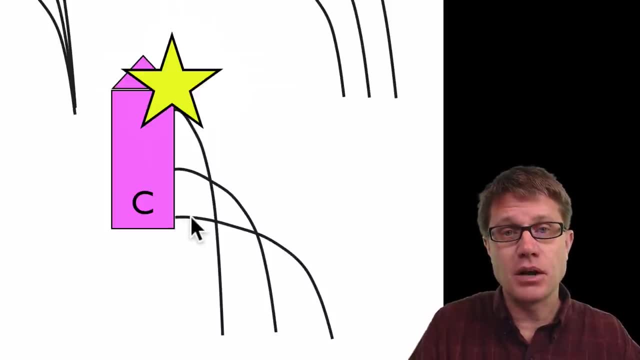 the streams are going to come out. Well, the correct answer is C. Why is that? It is because if we look down here at the bottom, this is like the second part of the pipe. So on the left side of the pipe we have way more potential energy inside the milk, And so that is going. 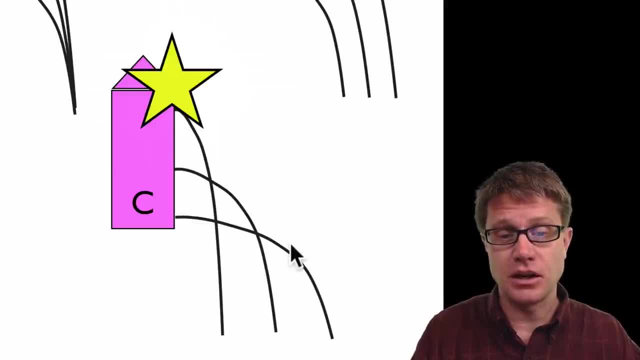 to be converted to more kinetic energy And the stream is going to go out farther, Whereas if we go to the top, it is not going to have as much potential energy above it And so it is not going to be able to have as much velocity, So it is not going to go out as 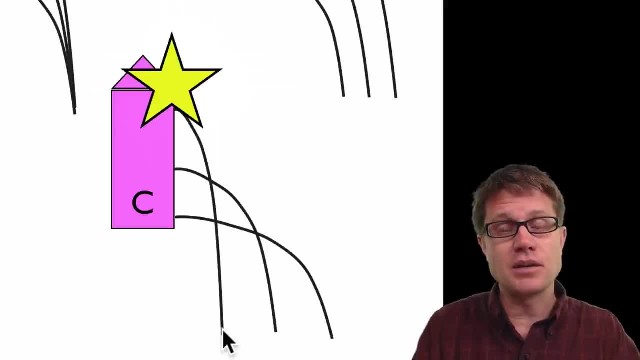 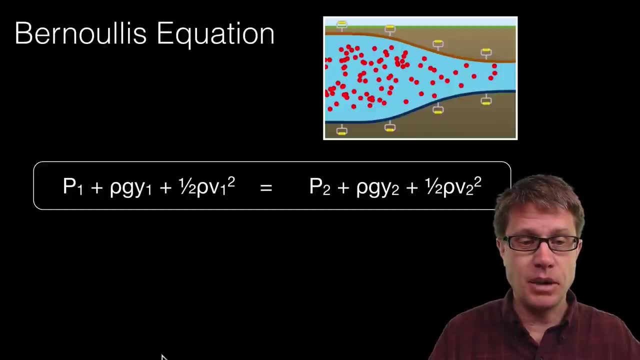 far, And so understanding both sides of the pipe. where is the potential energy greater? it really helps you understand how Bernoulli's equation works, And so it is written like this Left side: remember it is going to be the pressure energy. 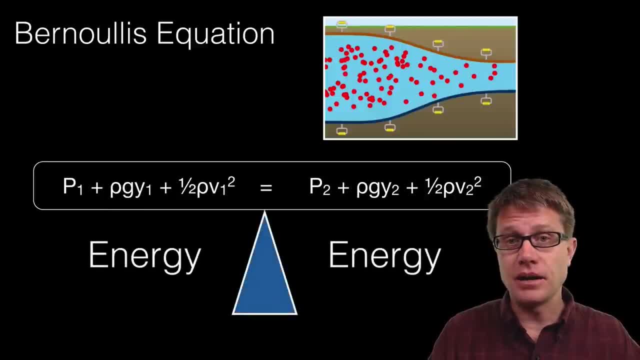 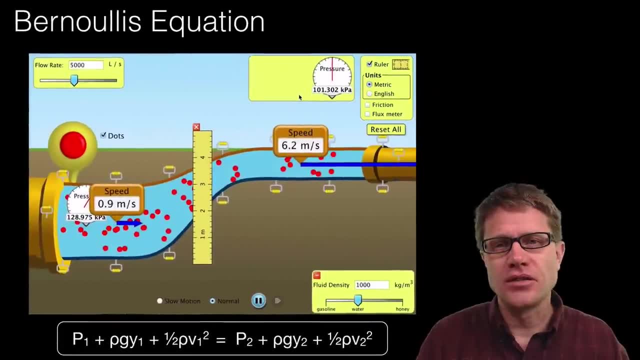 the potential energy and then the kinetic energy, And they are going to balance. So it is the conservation of energy. If we know what is on the left side, we can solve kind of for what is on the right side. So let's try to solve a problem using Bernoulli's equation. 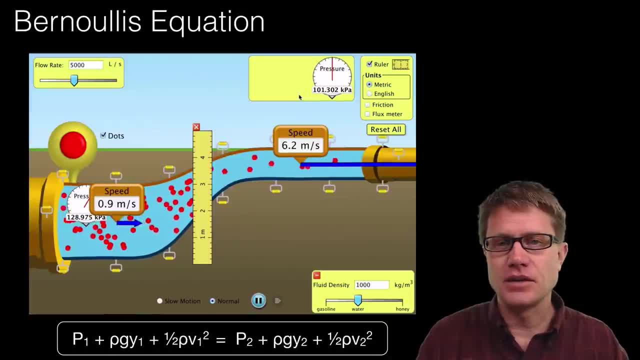 So I have got a pipe, I have got a left side and a right side. On the left side, you can see, the velocity is lower. I am giving you the pressure on the left side, But what we are going to solve for is the pressure on the right side. 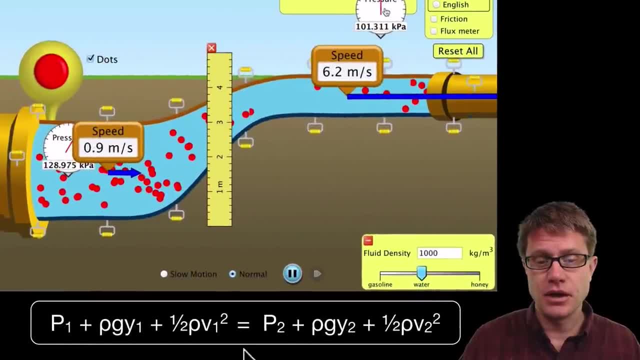 So let's go through this equation: On the left side, I am giving you the pressure On the right side, we do not know what that pressure is On the left side. do we have less or more potential energy in the pipe on the left side than we would on the right side? Well, the 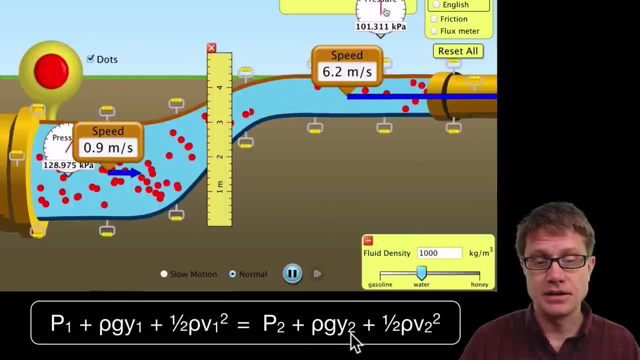 density of the fluid, since it is water, is going to be the same on both sides And since the pipe on the right side is going to have a higher height, it is going to have a higher potential energy on the right side. What about this? Are we going to have a higher kinetic? 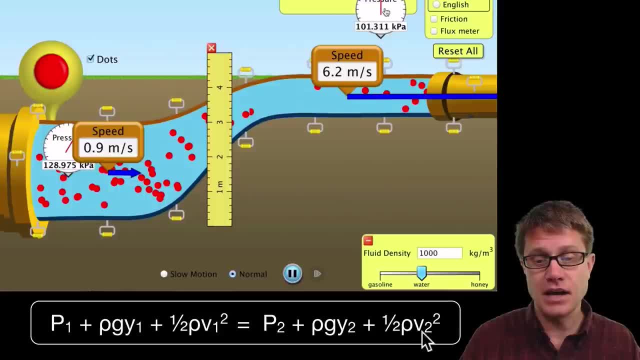 energy on the right side or the left side, Since the pipe on the right side is going to have a higher kinetic energy. since it is going faster on the right side, our velocity is faster on the right side- it is also going to have a faster kinetic energy or higher. 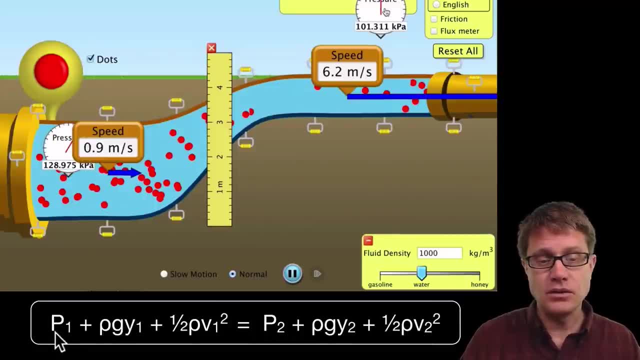 kinetic energy on the right side And since I am giving you the pressure on the left side as 128, we would expect to have a pressure on the right side that has to be lower, since we have higher potential and kinetic energy on the right side of the pipe. So let me show. 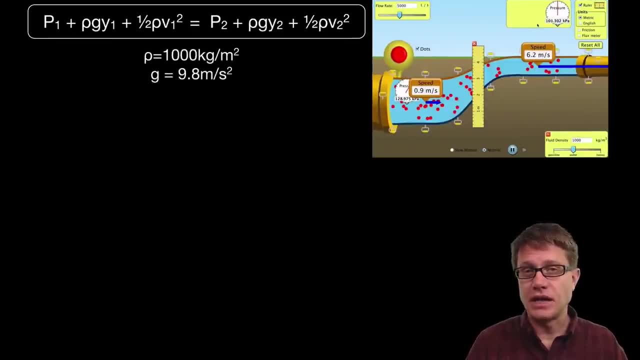 you how I would solve this. I would write it out with the things I know. So the density of the water, since it is the same fluid, is going to be 1000 kilograms per meter second, And we know the gravitational field strength is 9.8 meters per second squared On the left. 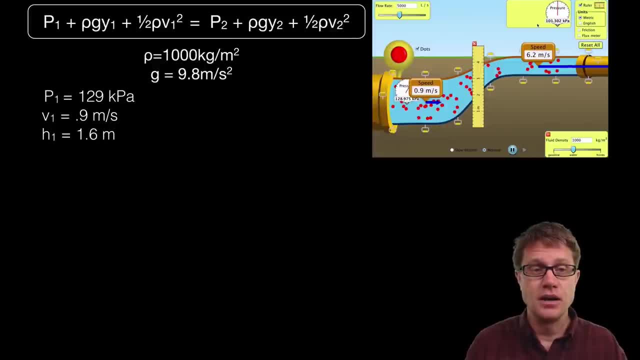 side of the pipe, we know the pressure- 129 kilopascals- We know the velocity and then we also know the height. And on the right side, what we do not know is going to be the pressure, That is the unknown. But on the right side again, we have a higher height. 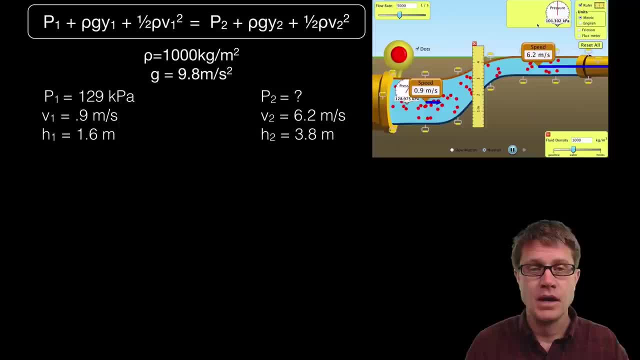 higher velocity, so we have higher energy right there. It should be a lower pressure. So if I were to write it out, I would write it out like this. Now, I am not going to include the units, because it simply would not fit on the screen. Watch one thing that could. 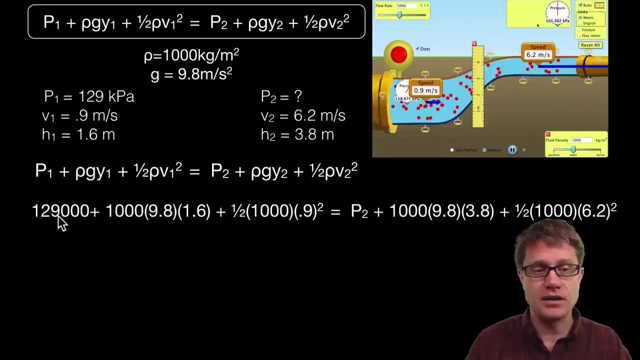 screw you up. Since it is 129 kilopascals, I am writing that out as 129,000 pascals, because that is the unit that we are going to use. I then solve it, And so this right here is going to be my potential energy left side, kinetic energy left side. If we compare that, 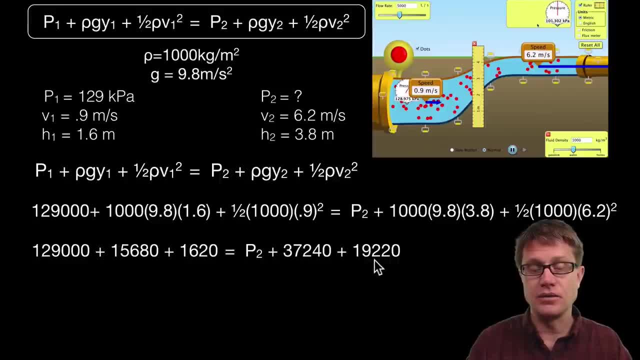 to potential and kinetic on the right side. you can see, on the right side both those values are greater, But we are simply solving for pressure 2. And so, using significant digits, I am getting around 90 kilopascals on the right side, And that is because I am limiting. 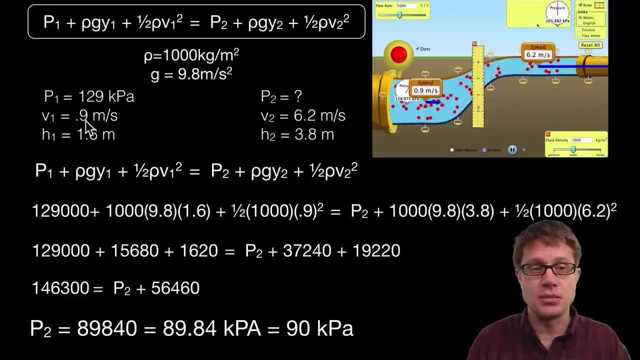 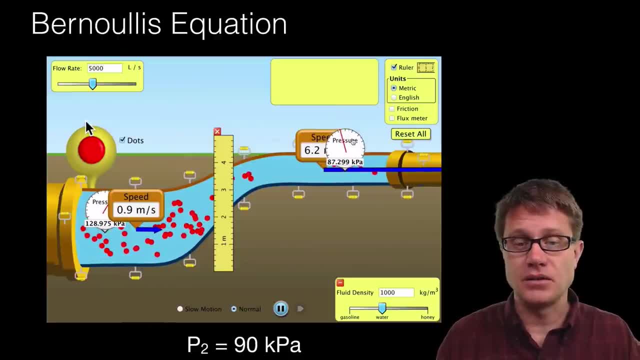 it by this: It is a low. it is not a very precise measurement in the velocity, So let's test that and see if that comes out. On the right side it is around 87 kilopascals, So it is around 90 kilopascals, And so we can use Bernoulli's equation not only to calculate. 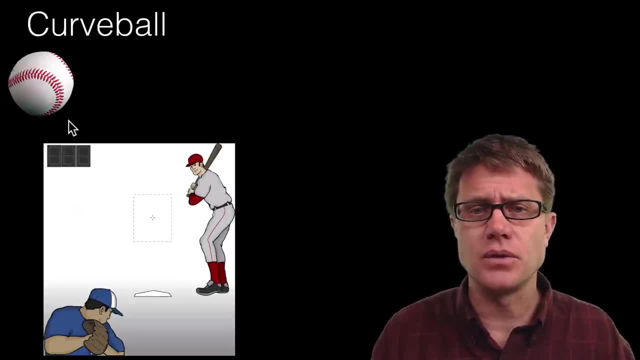 but we can use it to just analyze confusing situations when we have a fluid. So how does a curve ball work? When you throw a curve ball, it should drop. So as the pitcher tries to, or rather as the batter tries to, hit it, it is going to drop right at the end. And